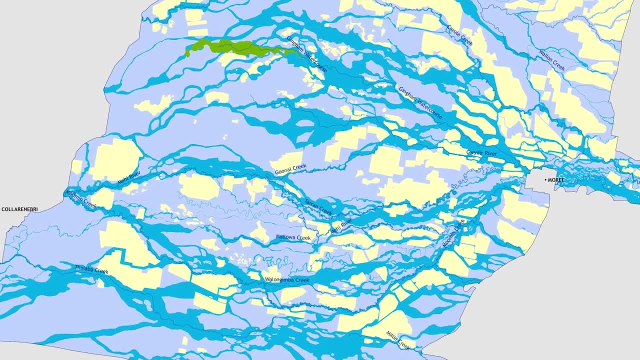 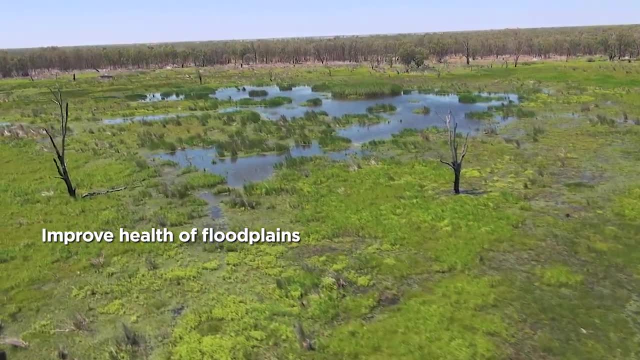 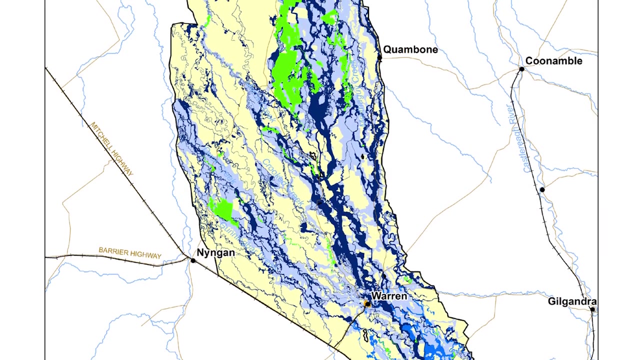 plans are providing for coordinated land use planning on a whole of valley basis. The Water Management Act 2000 requires that floodplain management plans identify the ecological and cultural benefits of flooding. Key outputs from floodplain management plans include a better understanding of the entire. 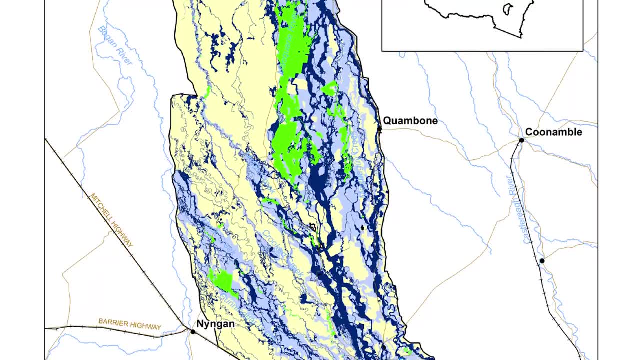 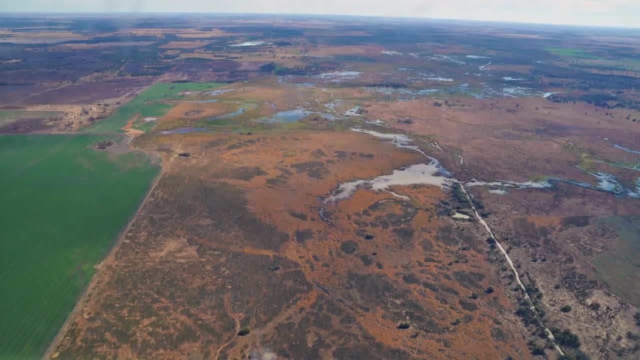 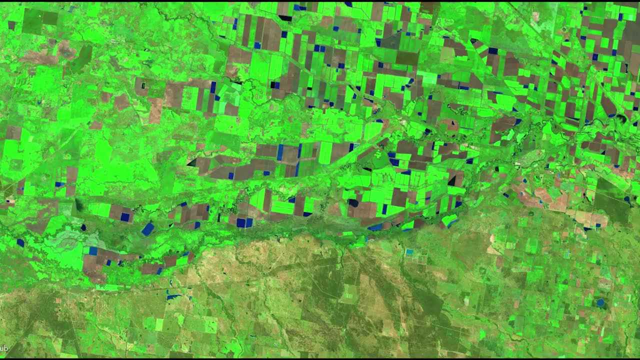 floodway network and the development of management zones. Management zones are areas that have common requirements for controlling flood work development and, together with the rules, provide the legal framework to assess and determine applications for flood work approvals under the Water Management Act 2000.. Using the latest technology and the best available data, we have a better 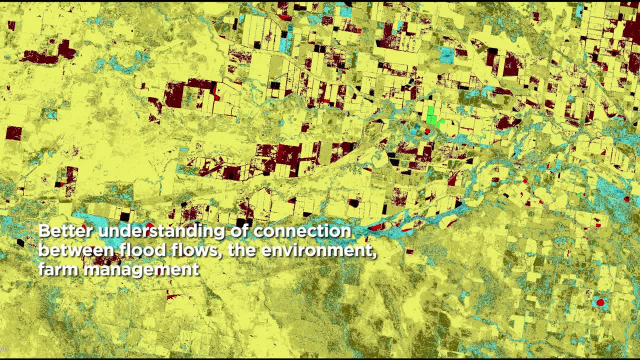 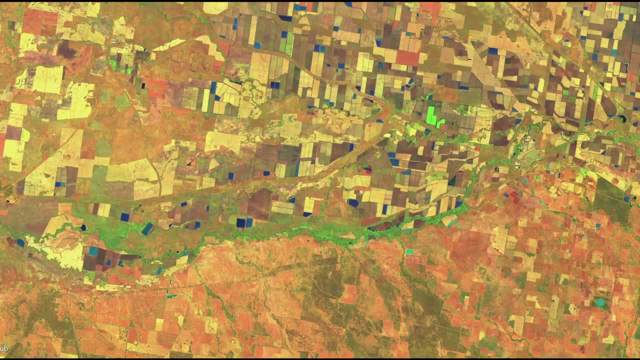 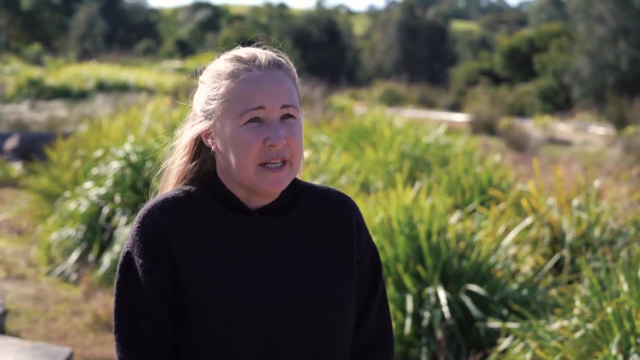 understanding of the connection between flood flows, the environment, farm management and risks to property and life. Understanding how our floodplains work means the Department and the community can plan with greater confidence. The first floodplain management plans to be developed will be in the Northern Inland Murray-Darling Basin. 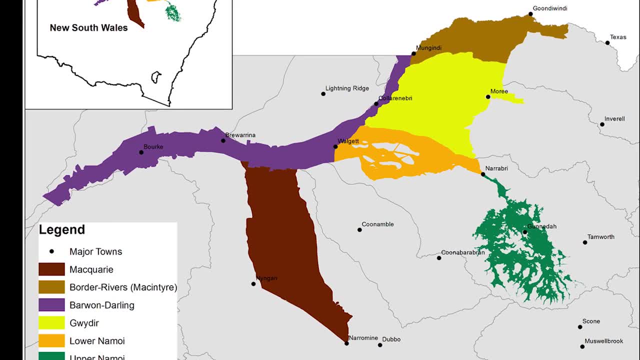 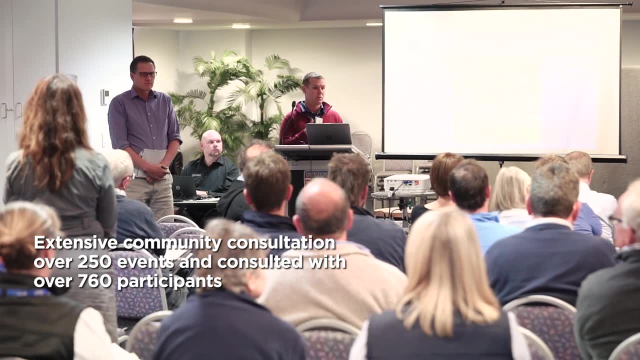 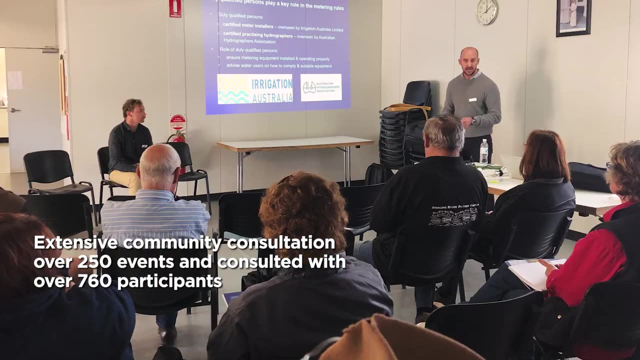 These valleys are the Macquarie, Namoy, Gwydir, Border Rivers and Barwon-Darling. The development of floodplain management plans has involved extensive community consultation. To date, the Department has facilitated over 250 events and consulted with over 760 participants, Balancing social, economic, environmental. 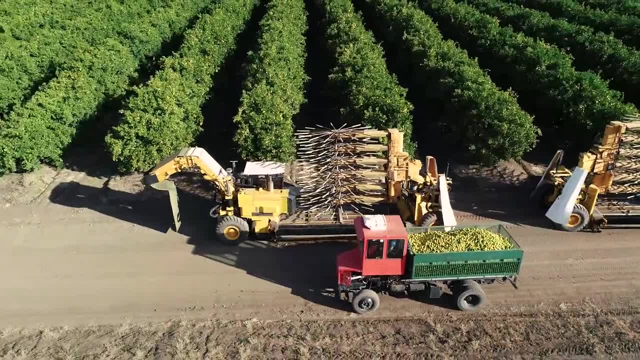 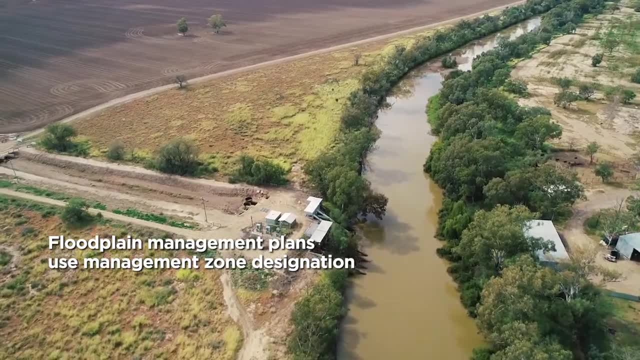 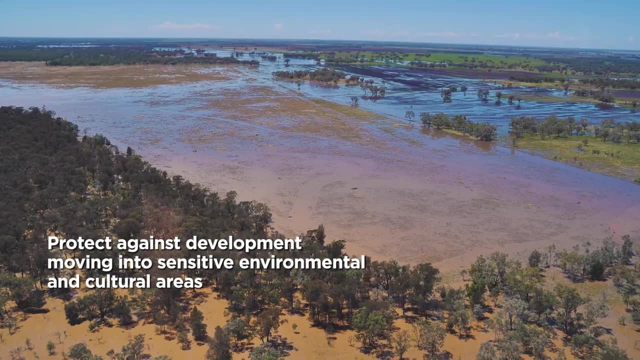 and cultural needs has been key in the development of floodplain management plans. Floodplain management plans use management zone designation with associated rules to control how and where flood works can be constructed or modified. Importantly, management zone designation and the associated rules protect against development moving into sensitive 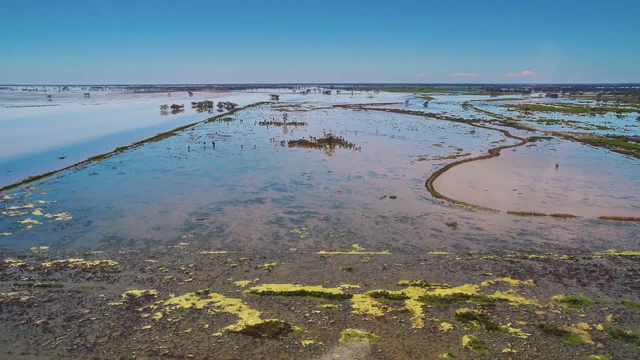 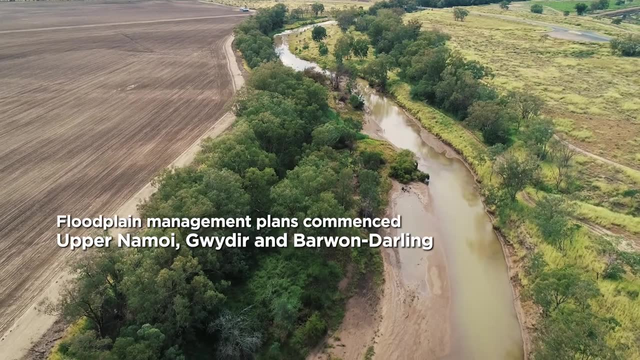 environmental and cultural areas, while recognising the need to manage the risk to life and property from the effects of flooding. Floodplain management plans have commenced for the Upper Namoy, Gwydir and Barwon-Darling. Floodplain management plans for the Lower Namoy, Border Rivers and Macquarie are: 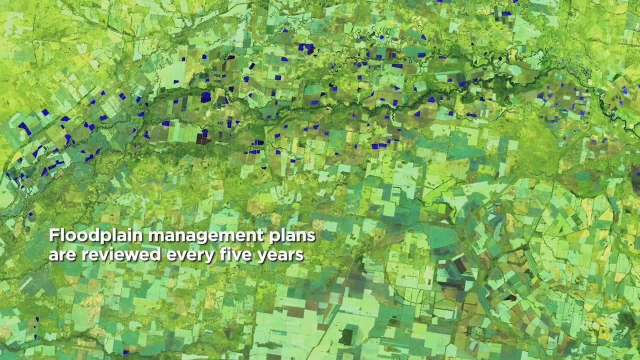 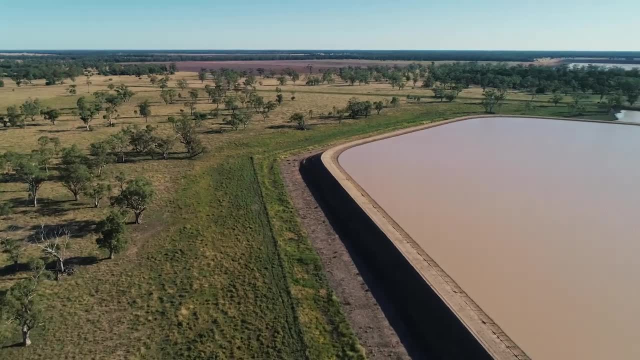 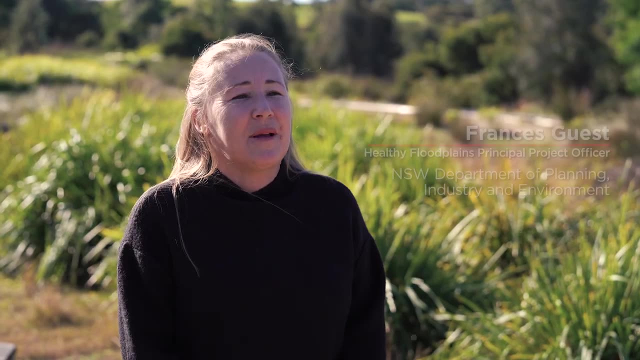 expected to commence by the end of 2020.. Floodplain management plans are reviewed every five years using the latest information and technology. If required and appropriate amendments can be made to the floodplain management plan following the review. Inclusive consultation is part of this review. Floodplain-